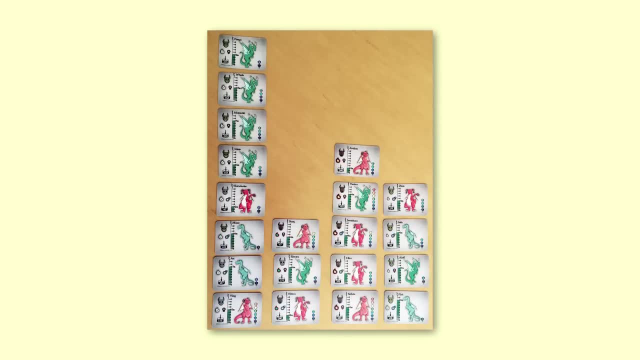 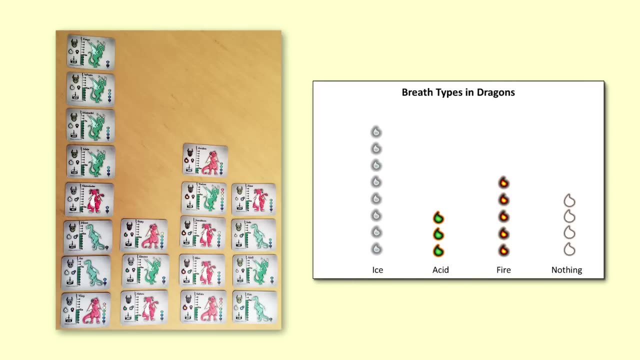 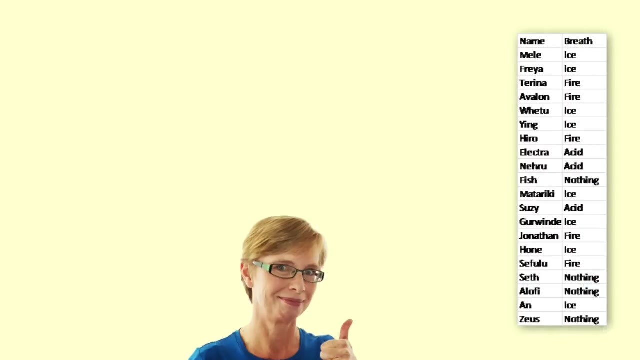 Another type of pictograph uses data cards. Each card shows the data for one individual person or thing. This pictograph shows us that we have more dragons that breathe ice than breathe acid fire or nothing special. The data for a pictograph is categorical. We are counting instances of a characteristic. 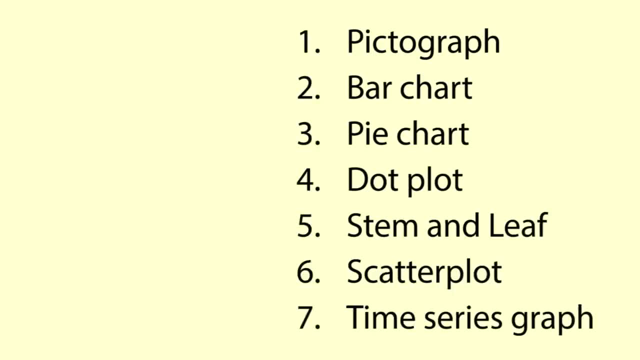 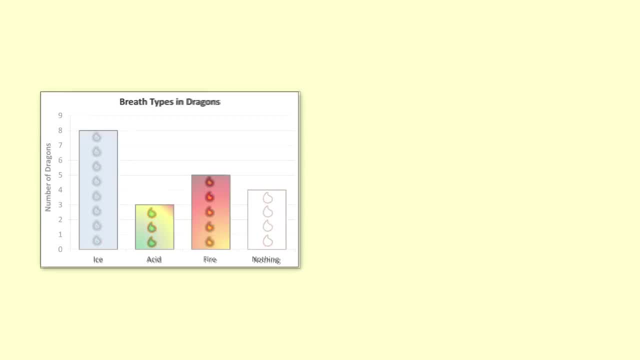 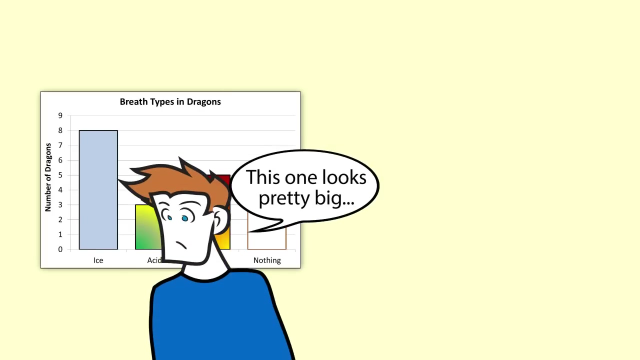 not measuring anything- Bar chart- This is also sometimes called a column chart. The data we showed in the pictographs can also be represented in a bar chart. In a bar chart, the length or height of the bar represents the number of times that object occurs, or the frequency. On bar charts it is easy to see which. 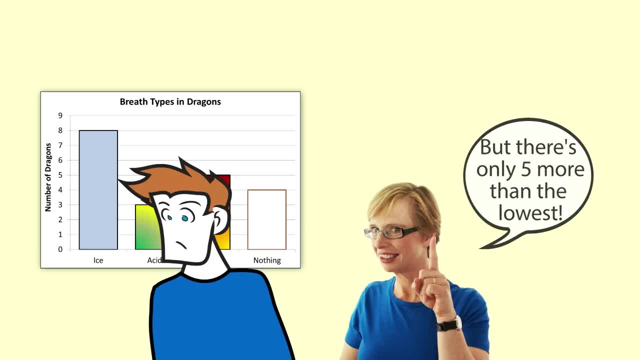 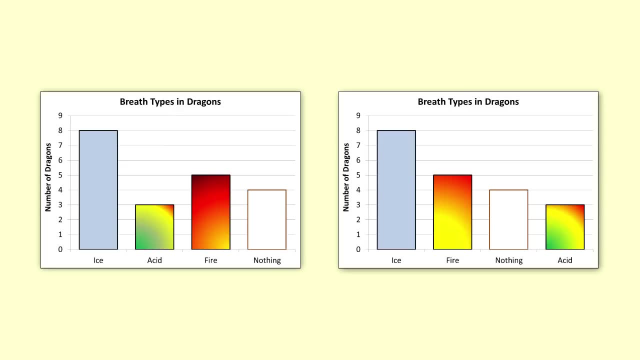 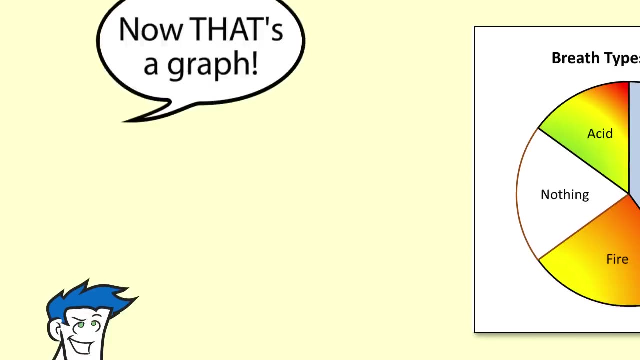 category is the target is the biggest, even when there is little difference. We can order the categories by size to give more information. Bar charts can be used for categorical data and for some numerical data, Pie charts. Pie charts are popular with non-statisticians. 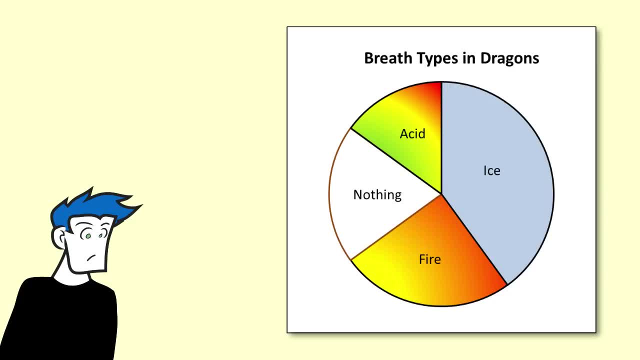 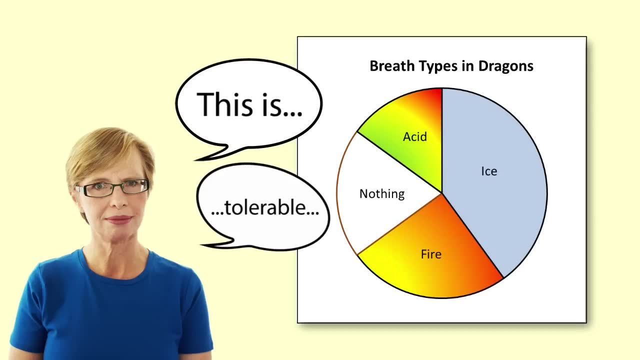 The area of each segment of the circle or pie represents the proportion for each of the categories. It is only acceptable to use a pie chart if you have five or fewer categories And the data is categorical and does not have an inbuilt order to it And you keep the graphs. 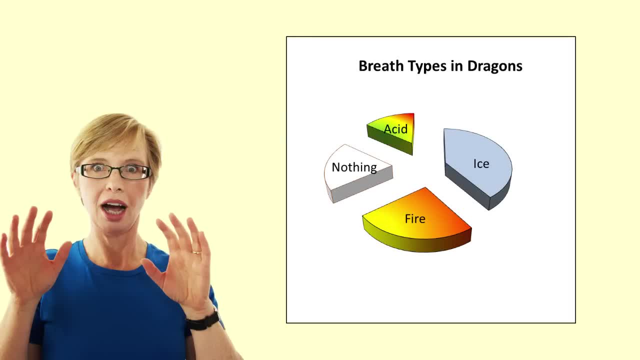 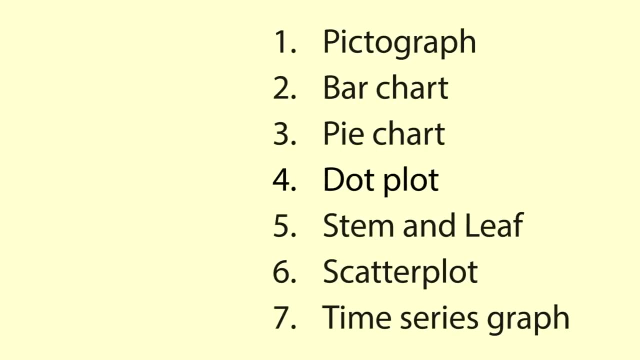 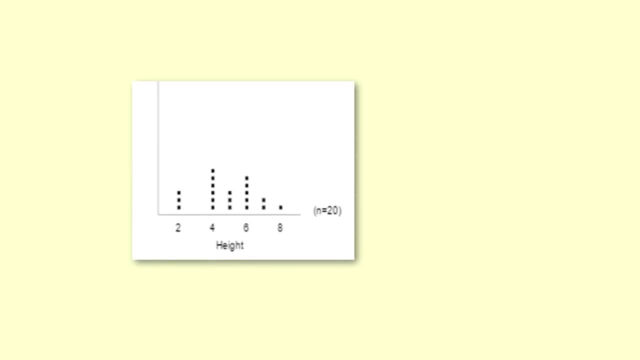 simple, no 3D and absolutely no exploding. People like pie charts, but they are only good in a few circumstances. Dot plots- Now dot plots are really useful. Dot plots are used for numerical data. Each dot represents one data point. In this dot plot of heights, each dot corresponds. 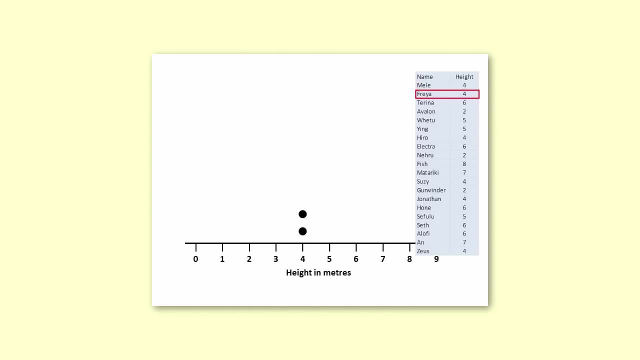 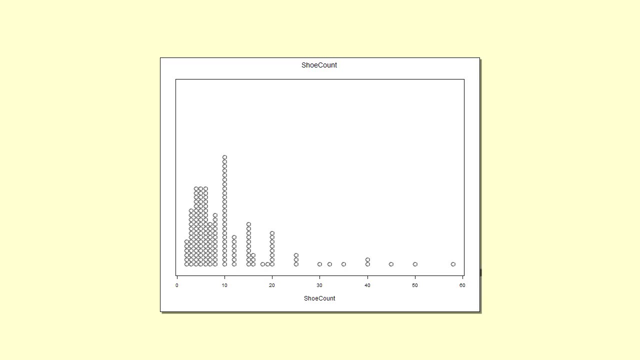 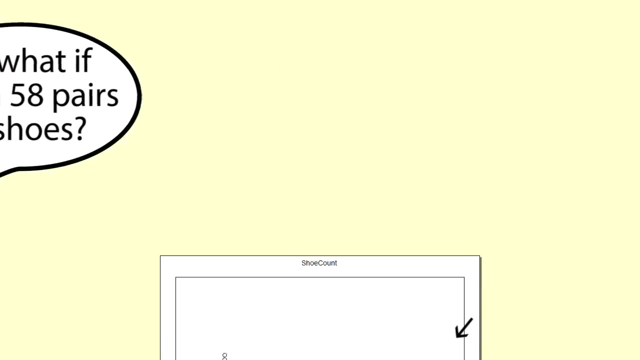 to one. dragon Dot plots are like number lines, but with the dots stacked up when there is more than one object that has the same value. This dot plot shows the number of pairs of shoes different people said they owned. Each dot represents one person. 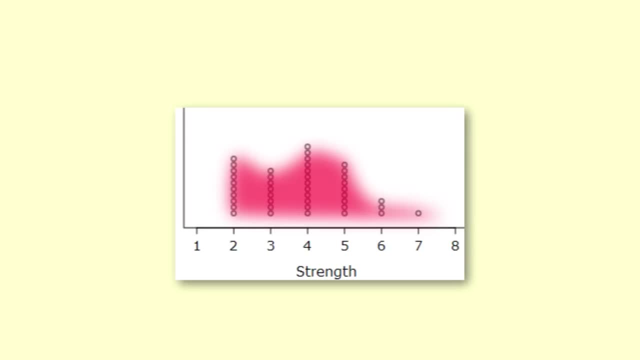 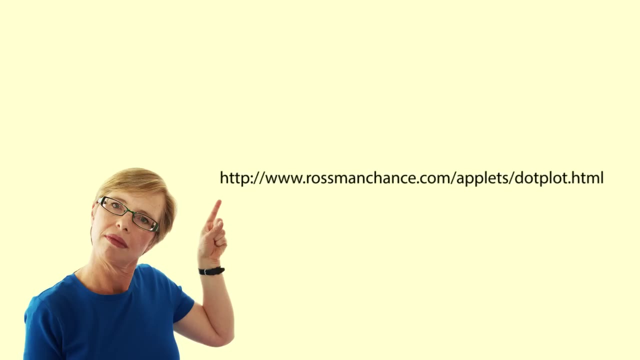 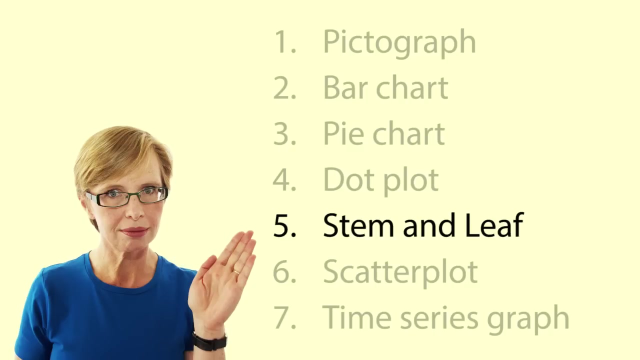 Dot plots are great for getting an idea of the shape of the distribution of the data. Mostly we use computers to make dot plots. This is a very good applet you can use for free. Stem and leaf plots. Stem and leaf plots are great for getting 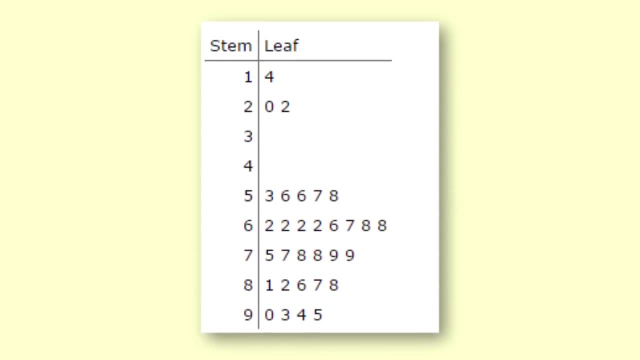 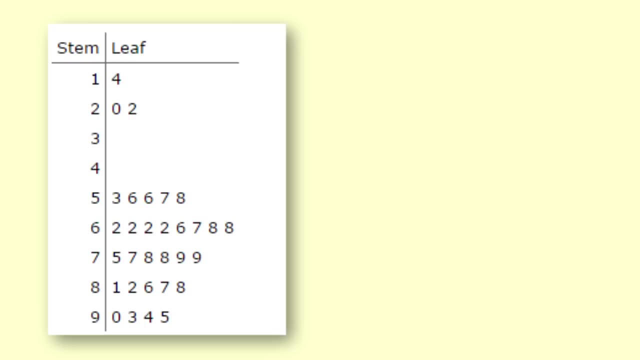 a quick idea of the shape of the data. The stem is the first digit of the number and the leaf is the second digit. This stem and leaf plot is of the grades a class of students got on a test out of a hundred. You can see that one person got fourteen. one person got 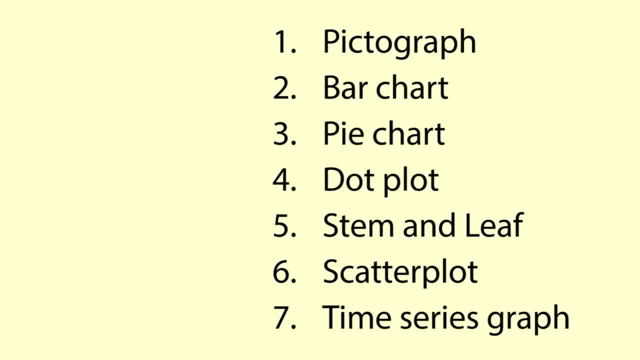 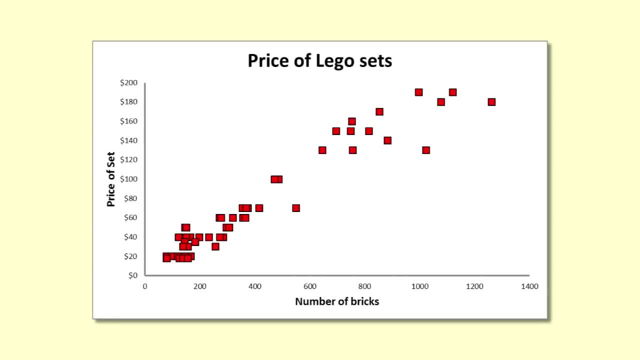 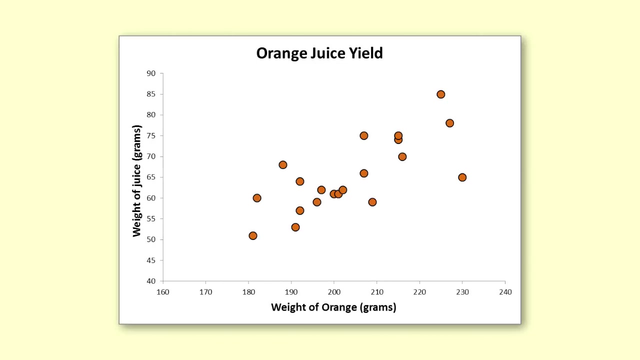 twenty and one got twenty-two. Scatterplot. Scatterplots are used for showing the relationship between two numerical variables. Each dot represents one observation or thing. In this case, each dot represents one set of Lego and shows the relationship between the number of pieces in this set and the price. In this example, we are looking at the relationship. 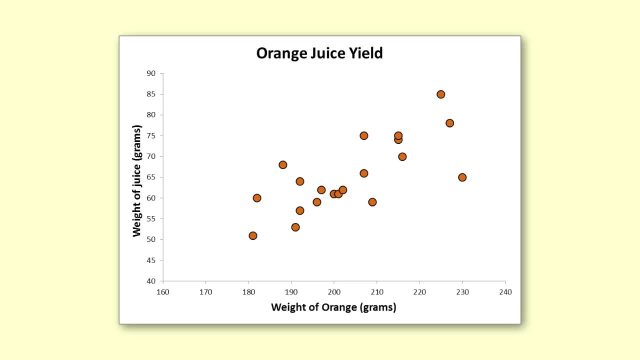 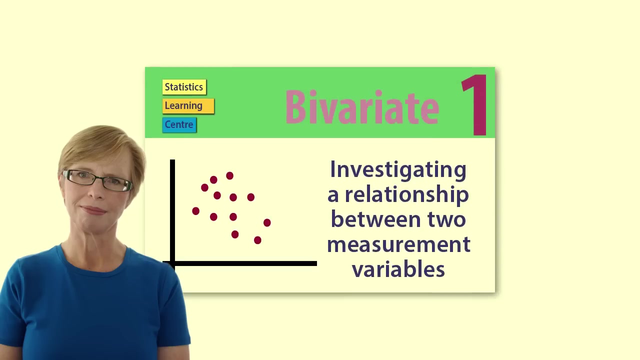 between the weight of an orange and the weight of juice it yields. Each dot represents one orange and its position corresponds to the weight of the fruit and the weight of the juice. You do not join up the dots in a scatterplot. You can see more about scatterplots in our video about scatterplots. 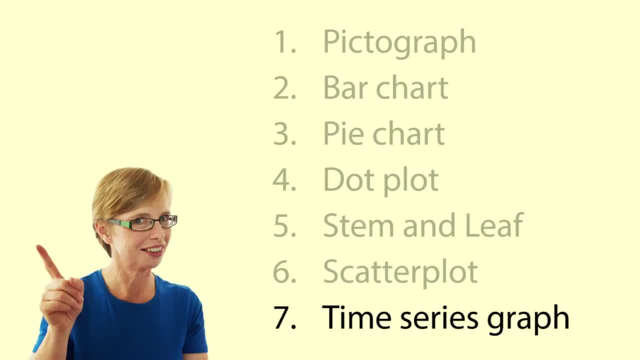 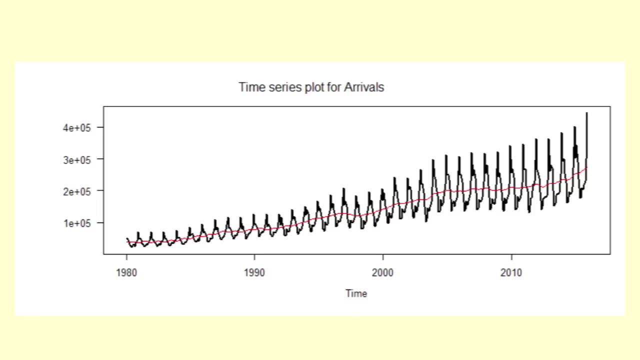 Time series plot. A time series plot is a special type of scatterplot. This time series plot shows the number of visitors arriving in New Zealand each month from 1980 to 2015.. The horizontal axis is always the in units of time equally spaced. there is one observation for each time value in: 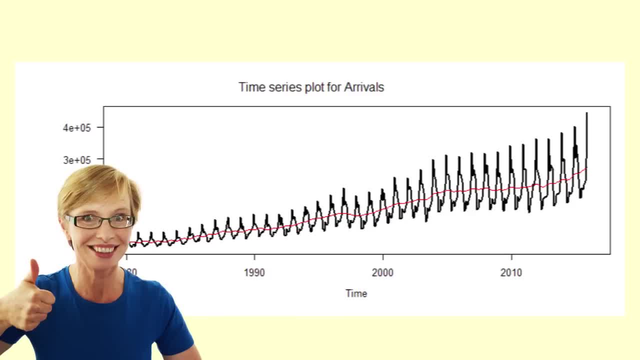 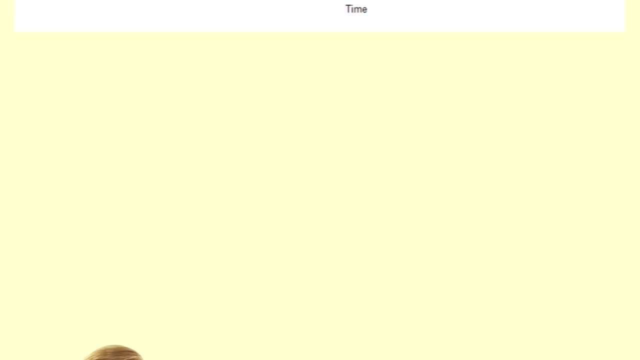 this case a month. it makes sense to join up the dots in a time series plot. you can see that there is a repeating pattern. you can see more about time series and time series graphs in our video understanding time series. there are other types of graphs as well, but we are not covering them in this video. the 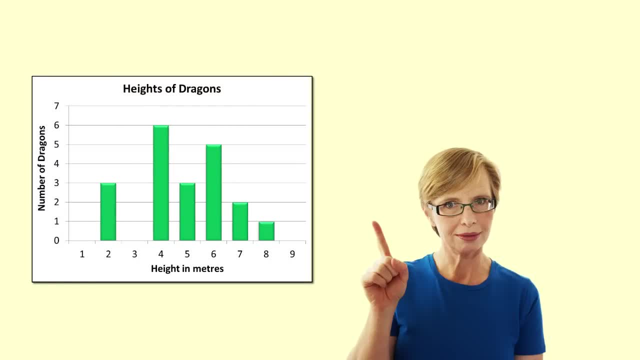 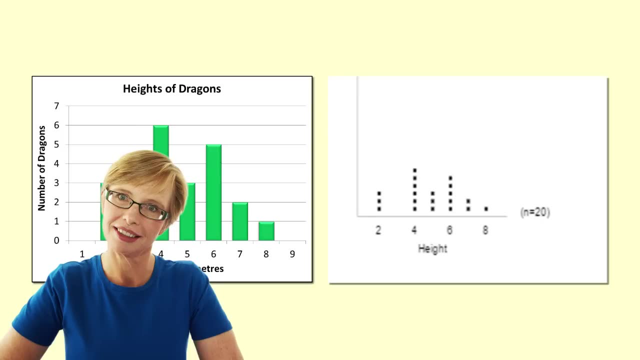 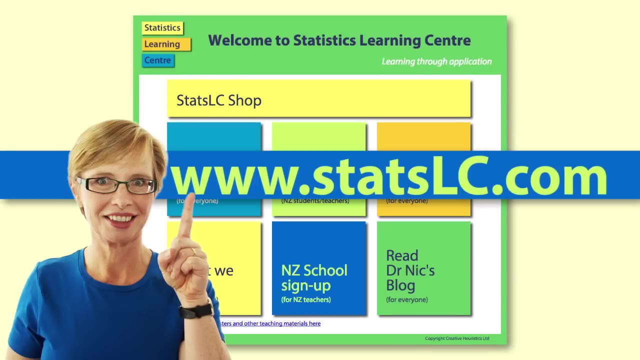 choice of graph depends on the context and purpose of our investigation. often, more than one type of graph is appropriate. good statistical packages will create appropriate graphs for your data. this video was brought to you by Statistics Learning Center. visit our website for more resources to help you learn.